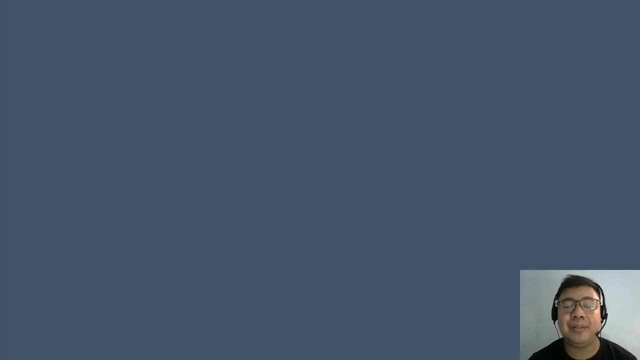 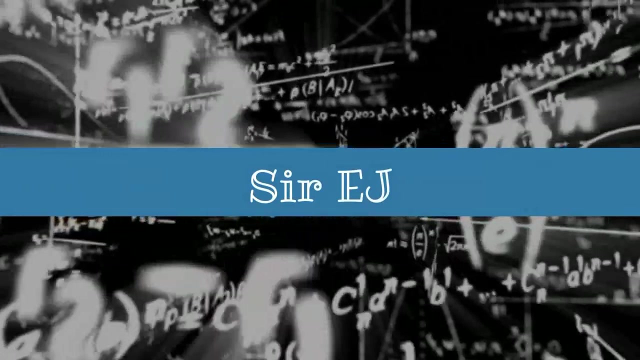 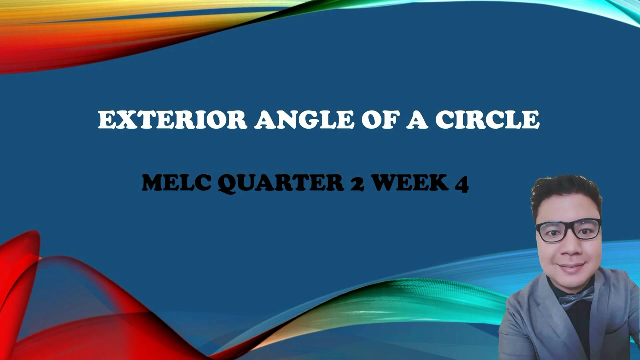 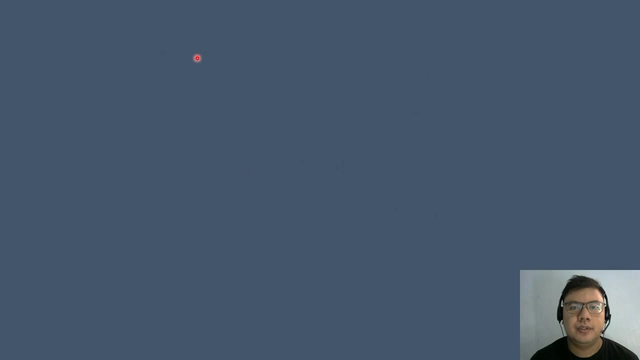 Hi guys, What's up? This is Sir EJ, and welcome again to another math tutorial. In today's topic, we will be discussing how to solve for the exterior angle of a circle. So let's have the following objectives in today's topic: 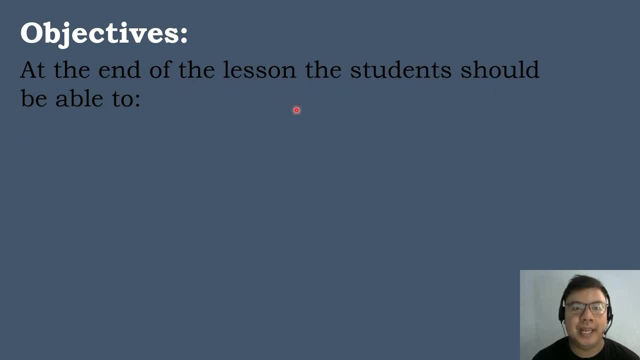 At the end of the lesson, the students should be able to: Letter A- Determine the relation among arcs and exterior angles of a circle. Letter B- Find the measure of arcs and exterior angles of a circle. And Letter C- Value accumulated knowledge as means of new knowledge. 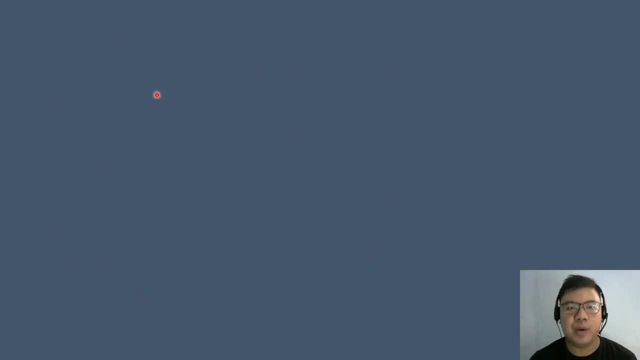 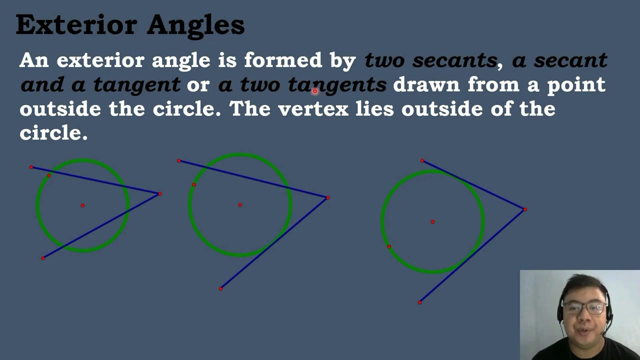 So let's define first what is an exterior angle. So when we say exterior angle, it is an angle which is formed by two seconds or a second and a tangent, or a two tangents drawn from a point outside the circle. then the vertex lies outside of the circle. 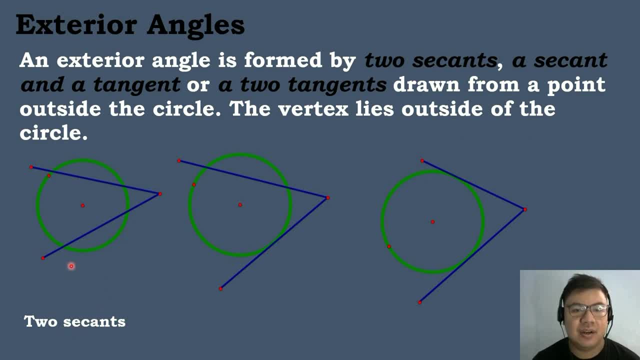 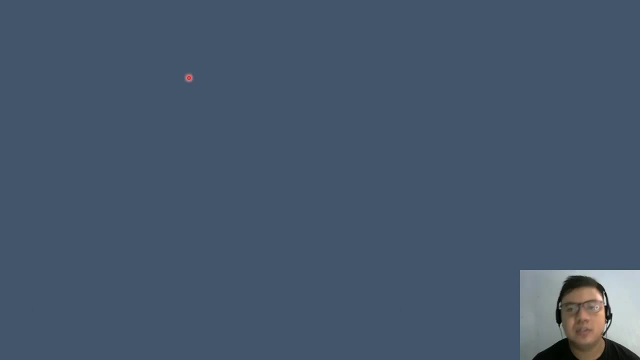 So on the first figure we have two seconds. On the second figure we have a second and a tangent, And on the third figure we have two tangents. So all of these three given figures are examples of exterior angles. 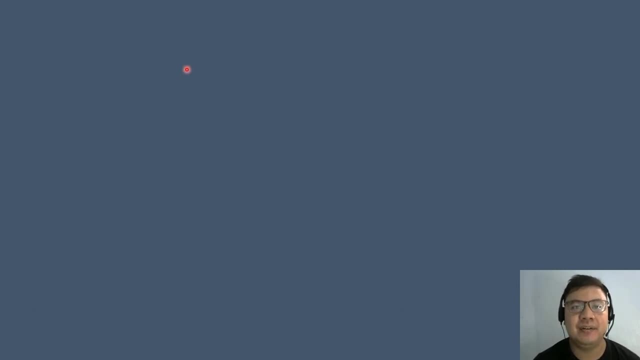 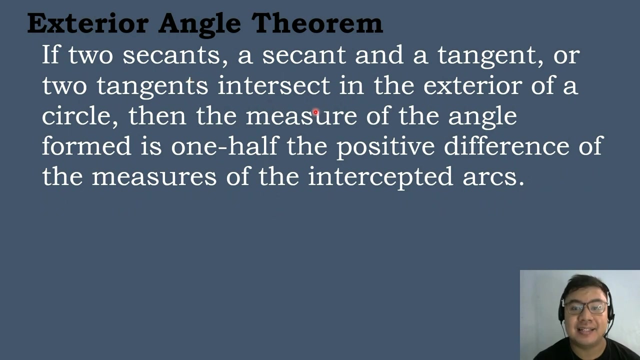 So after we have defined an exterior angle, let's now have the exterior angle theorem, wherein it states that if two seconds, a second and a tangent or two tangents intersect in the exterior of a circle, then the measure of the angle form is one half the positive difference. 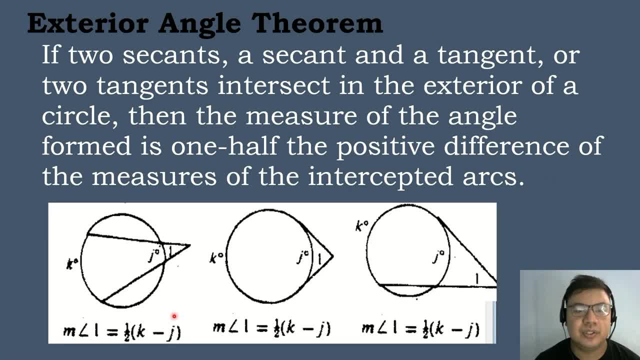 of the measures of the intercepted arcs. So the formula in finding the exterior angle will be: measure of angle one, or the exterior angle equals one half times the positive difference of the two intercepted arcs of the exterior angle. So the exterior angle is angle one and its two intercepted arcs is one half the positive difference of the two intercepted arcs of the exterior angle. So the exterior angle is angle one and its two intercepted arcs is one half the positive difference of the two intercepted arcs of the exterior angle. So the exterior angle is angle one and its two intercepted arcs is one half the positive difference of the two intercepted arcs of the exterior angle. 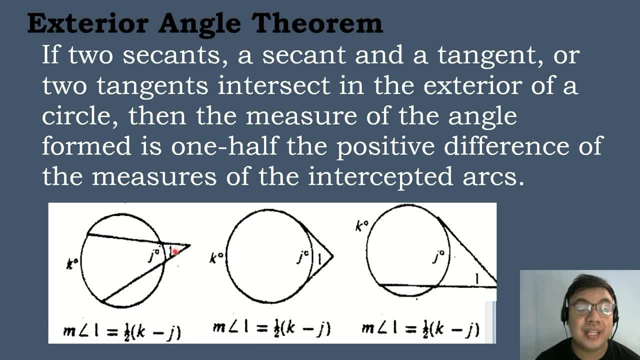 So the exterior angle is angle one and its two intercepted arcs is one half the positive difference of the two intercepted arcs of the exterior angle. exterior angle is angle 1 and its two intercepted arc is arc k and arc j, So we have the bigger arc. 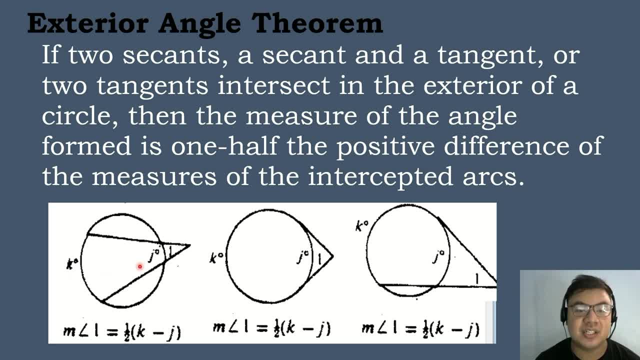 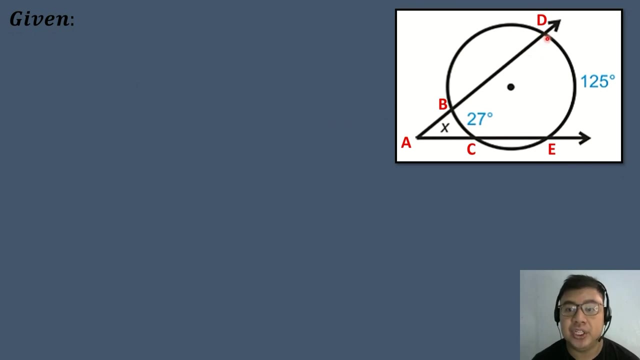 which is arc k, and the smaller arc, which is arc j. So our formula will be: measure of angle 1 is equal to one half times the quantity of the bigger arc, which is arc k, minus the smaller arc, which is arc j. So let's have our first example. So we have a given figure which is angle d, a, e. 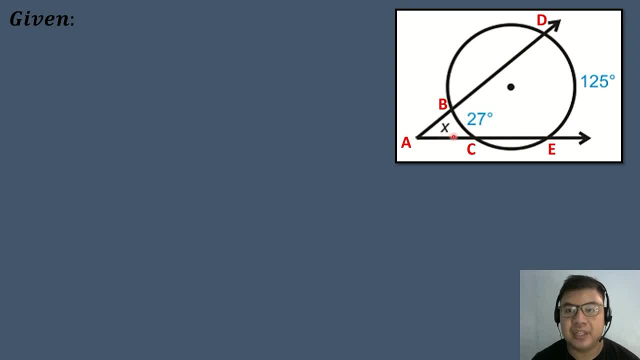 is the exterior angle, and then we have the two intercepted arcs, which is arc d e and arc b c. So arc b c is equal to 27 degrees, arc d e is equal to 125 degrees, and we have to find the measure of angle 1.. 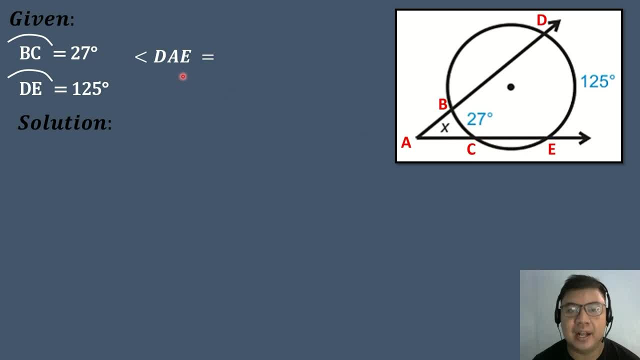 angle d, a, e, which is the exterior angle. So let's have the solution. So in our solution we will create our own formula according to exterior angle theorem. So we have the measure of the exterior angle, which is angle d, a, e is equal to one half times the quantity of the bigger arc. 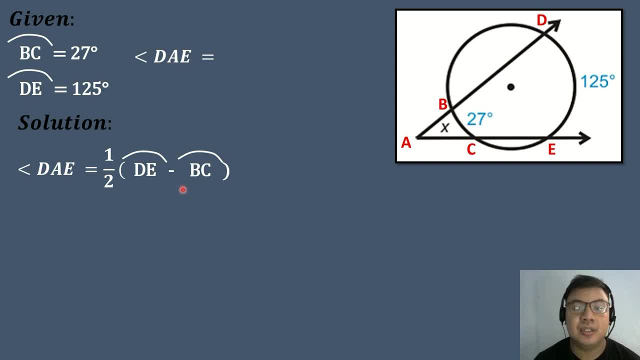 which is arc d e, minus the smaller arc, which is arc j. Then all we need to do is to substitute the given, So we will bring down angle d a. e equals. bring down one half times the quantity of the measure of arc d e is equal to 125 degrees. 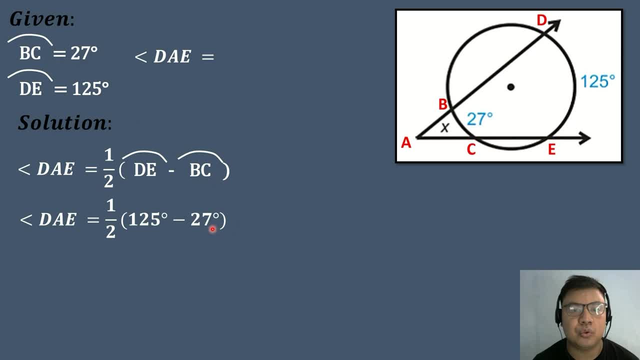 minus the measure of arc, b, c, which is equal to 27 degrees. Then again, bring down angle d, a, e equals, bring down one half, and then 125 degrees minus 27 degrees is equal to 98 degrees, and then the measure of angle dae is equal to one half. 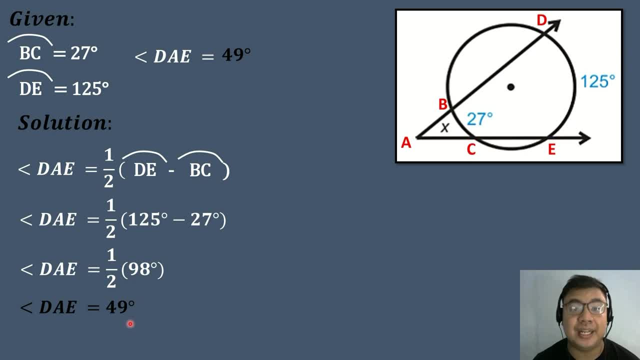 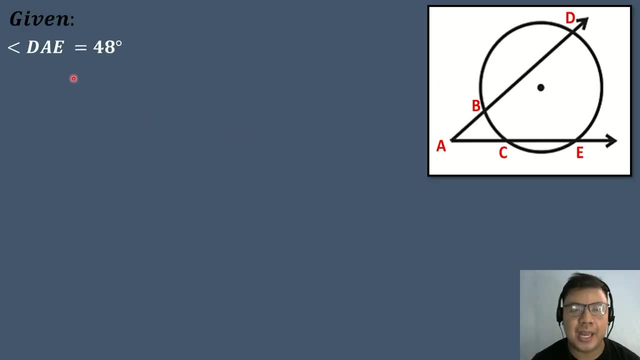 times 98 degrees is equal to 49 degrees. so angle dae, or the exterior angle of the circle, is equal to 49 degrees. so let's have our second example. so we have a given figure, so we have the measure of the exterior angle. angle dae is equal to 48 degrees. the measure of arc de is equal to 110. 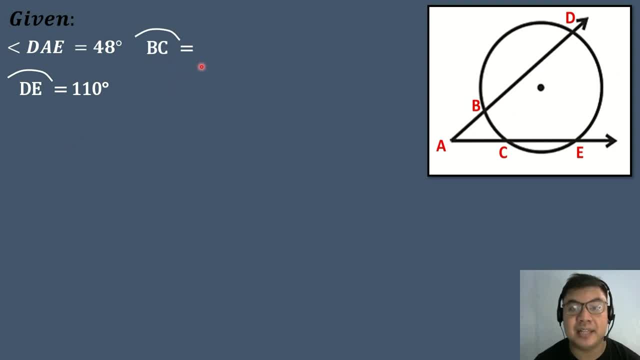 degrees, and the measure of arc bc is unknown, so let's have the formula. so we have angle dae. the exterior angle is equal to one half times the positive difference of the two intercepted arc of the exterior angle, which is the bigger arc, which is our d e, minus the smaller arc, which is arc bc. all we need to do is to substitute the given to arab. 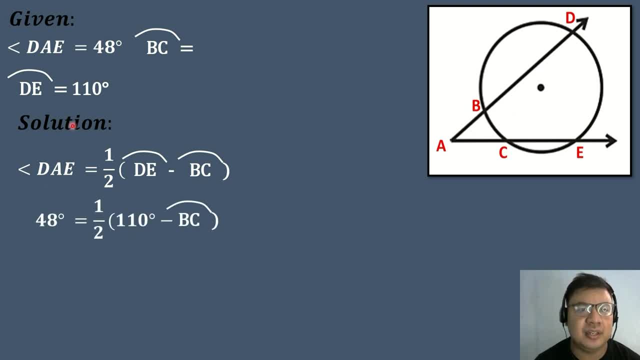 formula. so we have the measure of angle. dae is equal to 48 degrees, equals one half times the quantity of the measure of arc d e, which is equal to 110 degrees, minus arc bc, which is unknown. so we will write arc bc here and then after that bring down 48 degrees, and then we have the measure of. 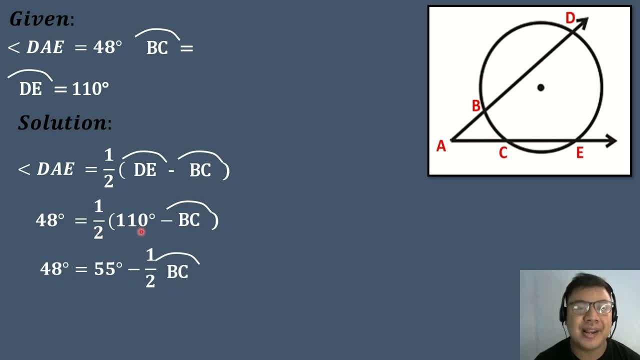 80 degrees equals one half times 110 degrees is equal to 55 degrees. then one half times negative arc bc is equal to negative one half arc pc. and then after that we will bring down 48 degrees, transpose 55 degrees positive 55 degrees, it will become negative. 55 degrees equals negative one. 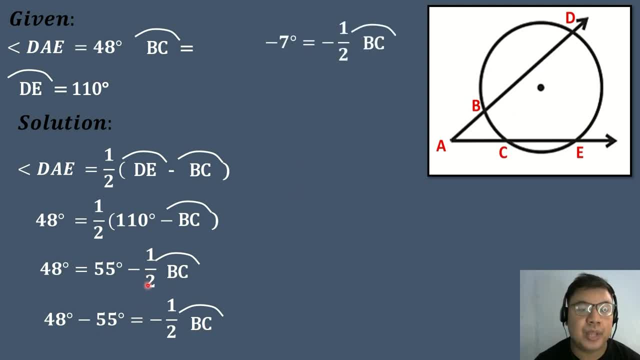 half arc bc and then after that we will add the equation and see what happens if we want to get an After that. we have 48 degrees minus 55 degrees is equal to negative 7 degrees. Equals: bring down negative 1 half arc PC. 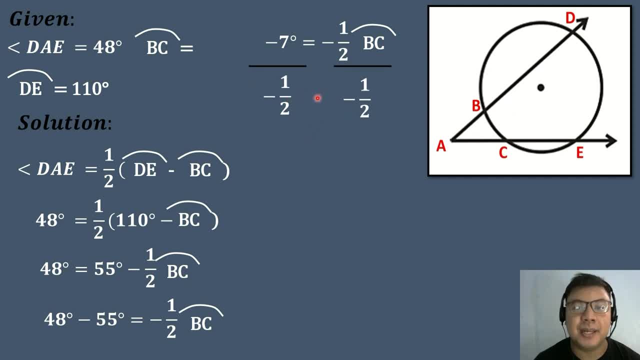 And then after that we will divide it both sides by negative 1 half to get the value of arc PC. So negative 1 half divided by negative 1 half will be equal to arc PC. And then negative 7 degrees divided by negative 1 half will be equal to 14 degrees. 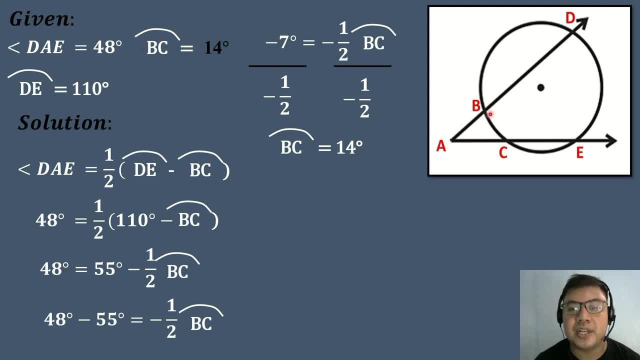 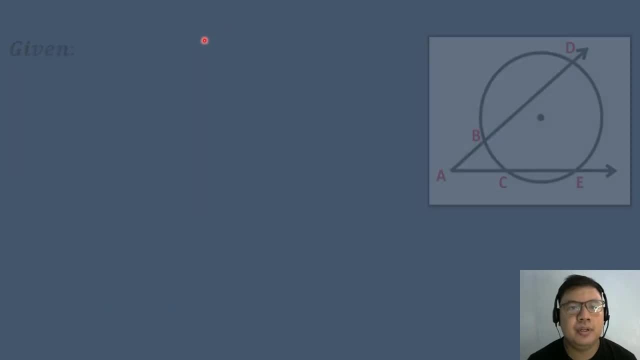 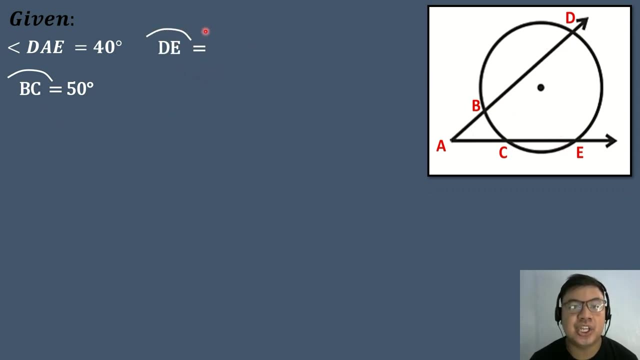 So the measure of arc PC, which is the smaller arc, is equal to 14 degrees. Okay, next let's have our third example. This time let's find the measure of our bigger arc. So let's find the measure of arc DA. 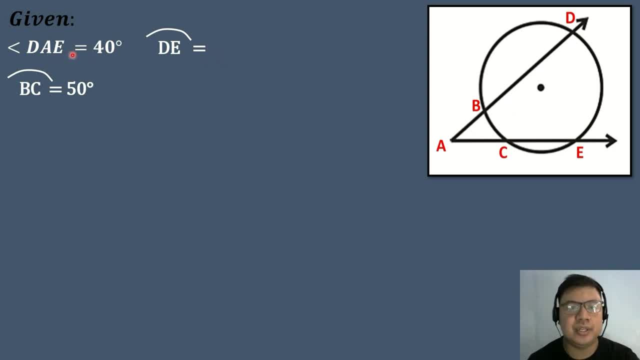 Given the measure of the exterior angle angle DAE is equal to 14.. The measure of the smaller arc, which is arc PC, equals 50 degrees. So let's now have our solution. So our formula will be: the measure of the exterior angle angle DAE is equal to 1 half times the quantity of the positive difference of the two intercepted arcs. 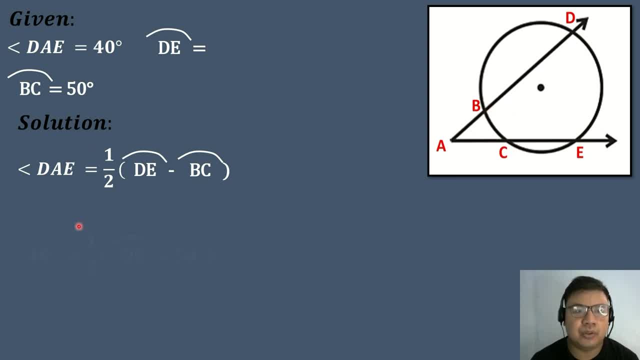 So angle DAE, the exterior angle, is equal to 40 degrees. equals: bring down 1 half. Then bring down 1 half times the quantity of arc DAE, which is unknown, so we will copy: arc DAE minus the bigger arc, which is arc BC, is equal to 50 degrees. 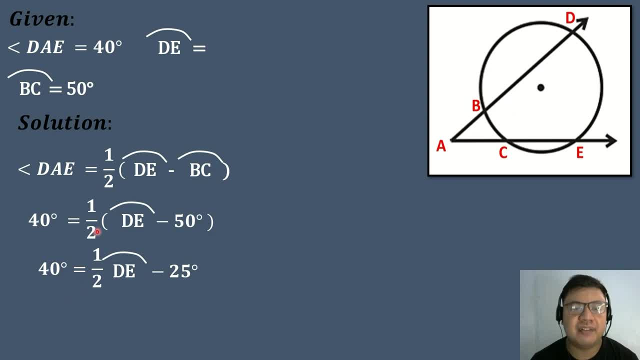 And then bring down 40 degrees equals 1 half times arc DAE, will be equal to 1 half arc DAE. And then 1 half times negative. 50 degrees is equal to negative 25 degrees. And then again bring down 40 degrees, then negative 25 degrees. 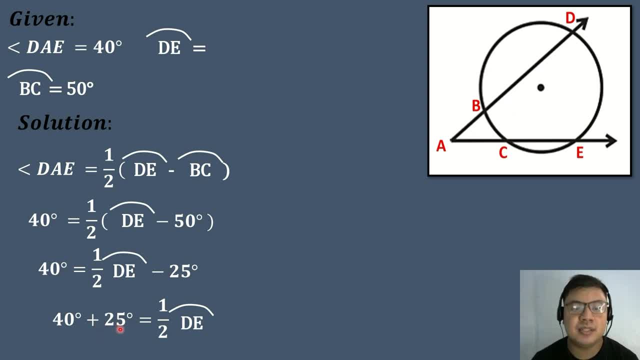 Transpose it will become positive. 25 degrees equals bring down 1 half arc DAE And then after that you will add 40 degrees plus 25 degrees. that will be equal to 65 degrees equals 1 half arc DAE. 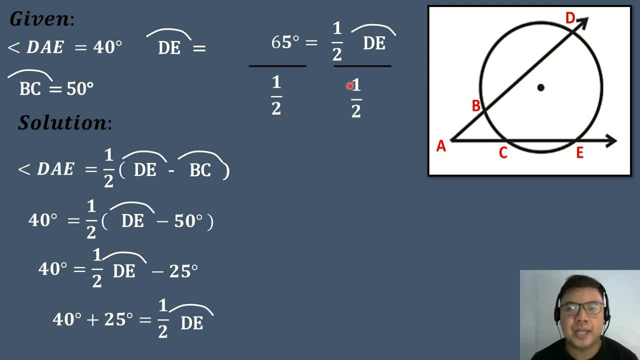 And then we will divide it both sides by 1 half to get the measure of arc DAE or the bigger arc. So 1 half divided by 1 half will be equal to arc DAE, And then 65 degrees. 65 degrees divided by 1 half will be equal to 130 degrees. 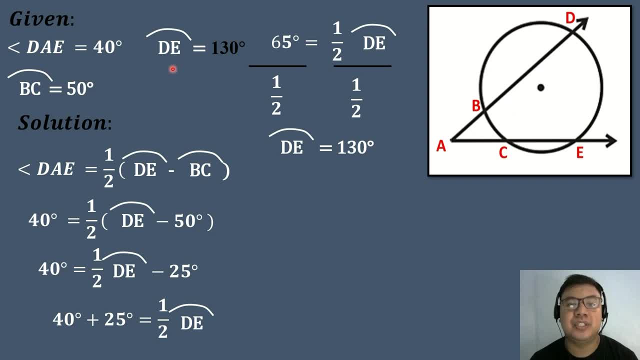 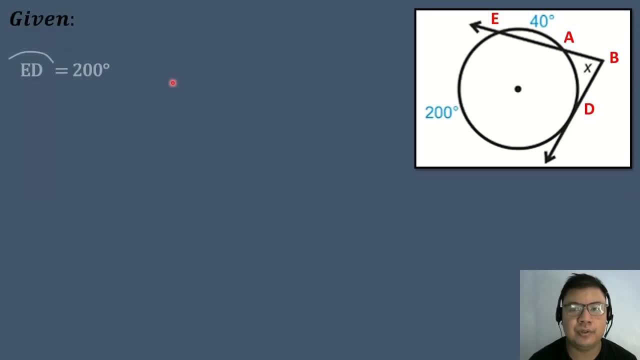 So the measure of the bigger arc, which is arc DAE, is equal to 130 degrees. So let's have our next example. So we have a given figure. So the measure of arc ED, which is the bigger arc, is equal to 200 degrees. 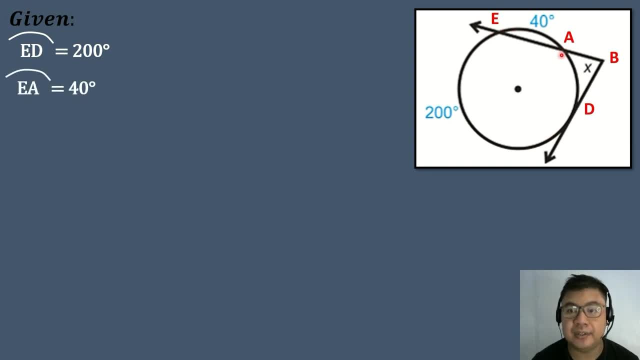 Then the measure of arc EA. this arc is equal to 40 degrees. And then let's find the measure of angle EVD, which is the exterior angle of the circle. So let's have our solution, So we will construct our formula to find the measure of the exterior angle. 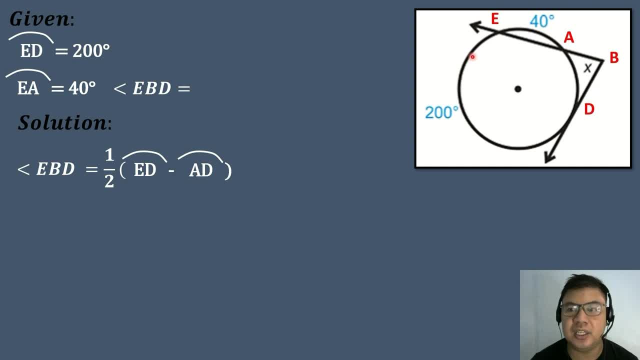 So the measure of the exterior angle angle EBD equals 1 half times the positive difference of the two intercepted arcs, which is arc ED minus arc AD. But before we can compute for the measure of the exterior angle we need to solve first for the measure of arc AD. 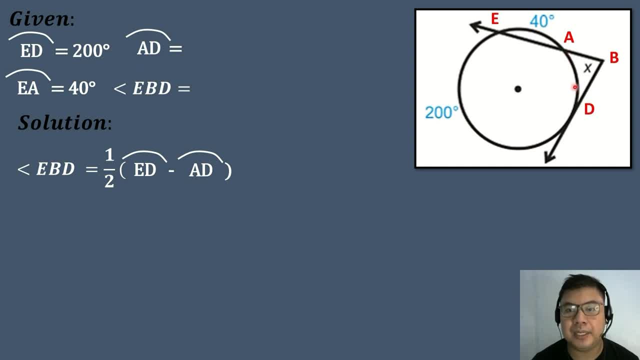 So the measure of arc AD will be equal to 360 degrees, minus the measure of arc ED, plus the measure of arc EA. So 200 degrees plus 40 degrees will be equal to 240 degrees. Then, remember, the measure of the circle is equal to 360 degrees. 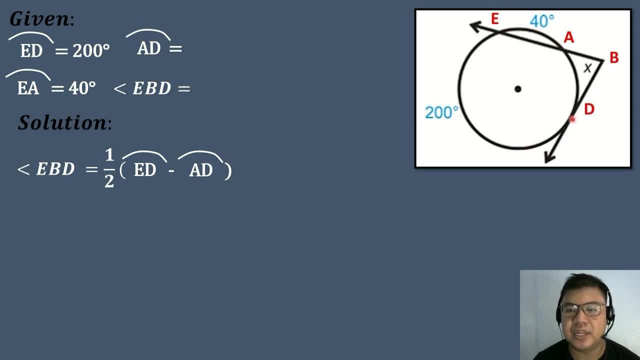 So we need to subtract this part of the circle, which is equal to 240 degrees minus the whole part of the circle, So 360 degrees minus 240 degrees will be the measure of arc AD, and that is equal to 120 degrees. 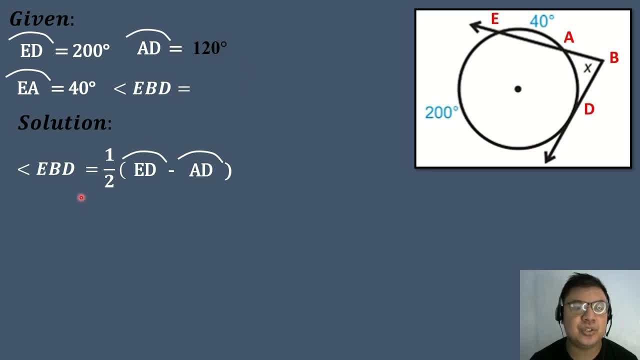 And then after that we will substitute the values. So the measure of angle EBD is unknown. Equals: bring down 1 half. Bring down 1 half times the quantity of the bigger arc, which is arc ED, is equal to 200 degrees minus the measure of arc AD is equal to negative 120 degrees. 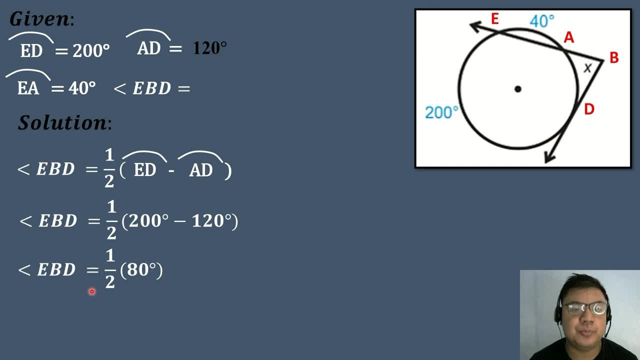 Bring down angle EBD equals: bring down 1 half and then 200 degrees minus 120 degrees is equal to 80 degrees, And then 1 half times 80 degrees is equal to 40 degrees. So the measure Of angle EBD is equal to 40 degrees. 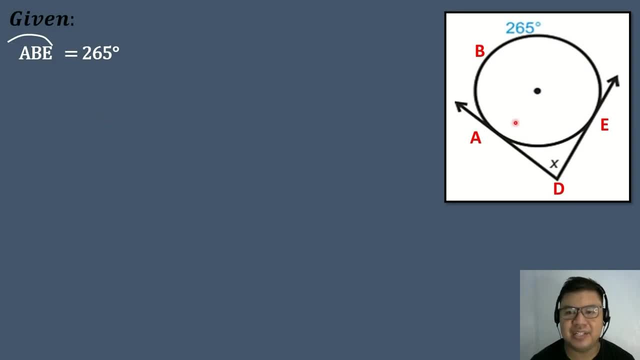 So let's now have our next example. So we have a given circle, So the measure of the bigger arc is equal to 265 degrees, And then we need to find the measure of arc AE. So the exterior angle is formed by two tangents. 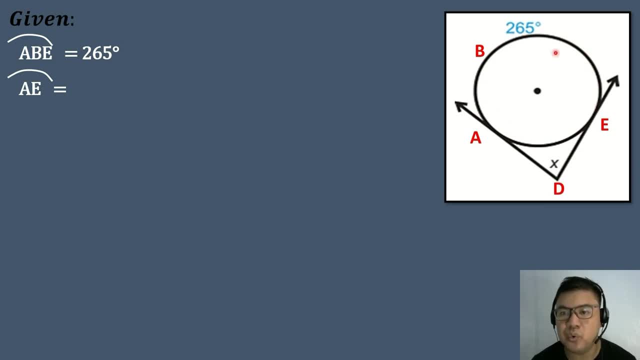 So if this arc, arc ABE is equal to 265 degrees, then to get the measure Of Arc AE, we will subtract 265 degrees by the measure of a circle which is equal to 360 degrees. So subtracting that 360 degrees minus 265 degrees will be the measure of arc AE, which is equal to 95 degrees. 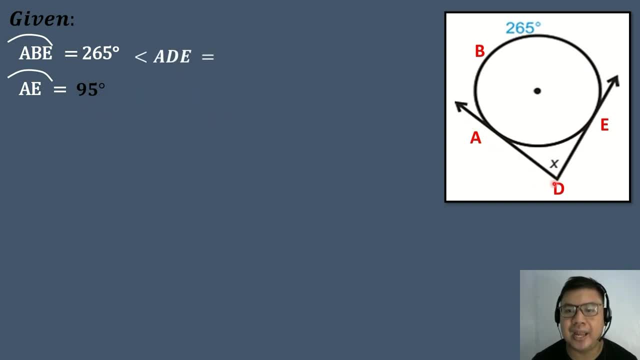 And then now we can compute for the measure of the exterior angle, which is angle ADE. We will use the formula: Angle ADE equals 1, half times the positive difference of the two intercepted arcs, which is arc ABE- the bigger arc- minus arc AE, which is the smaller arc. 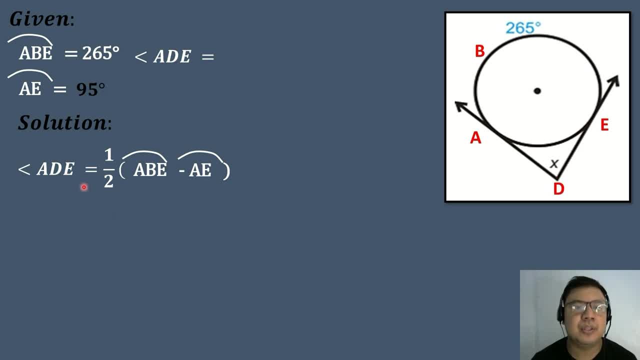 Then we will substitute the corresponding value. So the measure of angle ADE is unknown- equals 1: half. bring it down and then times the quantity of the measure of the bigger arc, which is equal to 265.. 265 degrees minus the Masher of the smaller arc, which is equal to. 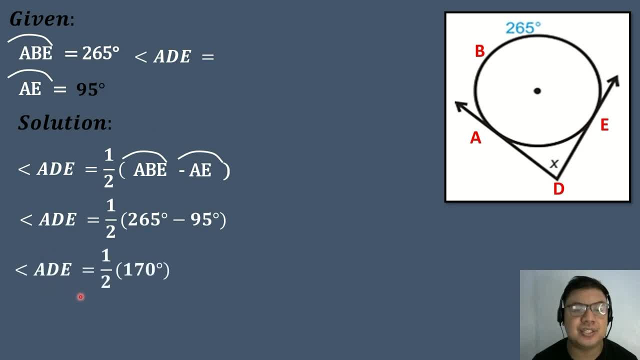 95 degrees, And then Angle ADE is equal to 1 half a. 265 degrees minus 95 degrees is equal to 170 degrees, and Then 1 half times 170 degrees is Equal to 85 degrees or the выше of the exterior angle. angle DD. 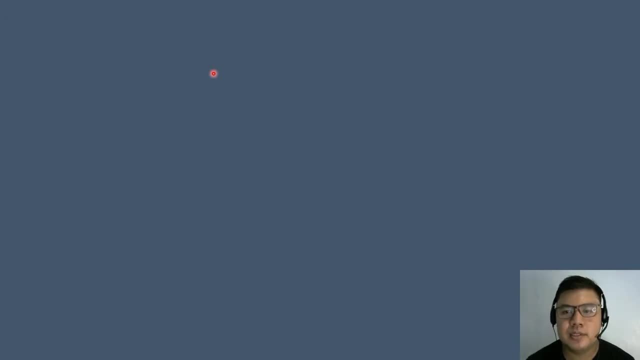 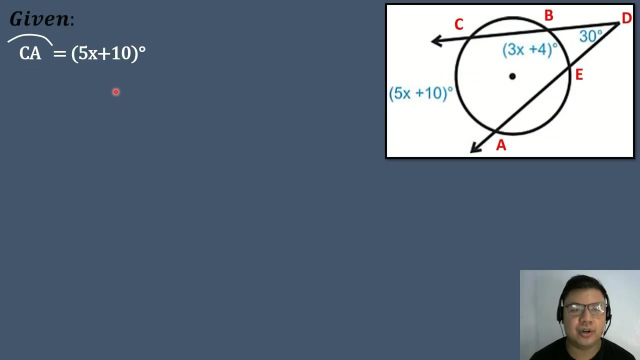 is equal to 85 degrees. so let us now apply algebra with our topic. so we have a given circle. so the measure of arc ca is equal to 5x plus 10, the measure of arc be is equal to 3x plus 4 and the measure of the exterior angle angle, cda, is equal to 30 degrees. so we need to find the. 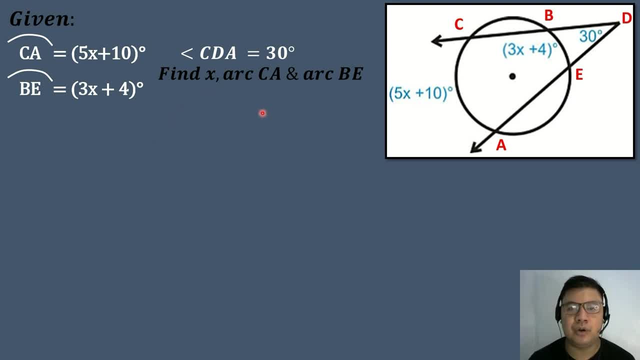 measure, or the value of x, the measure of arc ca and the measure of arc be. so let's construct now our formula. so the formula will be: angle cda, which is the exterior angle, equals one half times the positive difference of the two intercepted arc, which is arc ca minus arc be. then we will substitute. 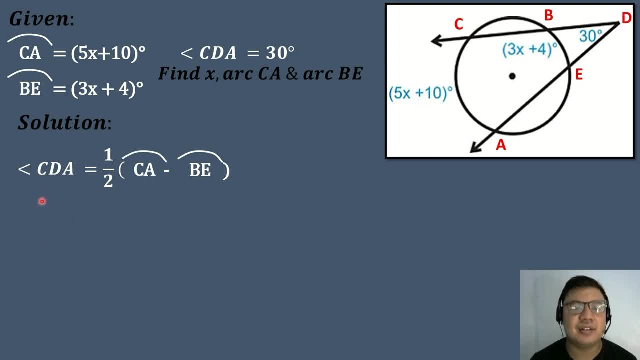 the corresponding value. so the value of angle cda is equal to 5x plus 10. the measure of arc cda is equal to 3x plus 10. the measure of arc be cda is equal to 30 degrees equals one half times the quantity of the value of arc ca, which is the 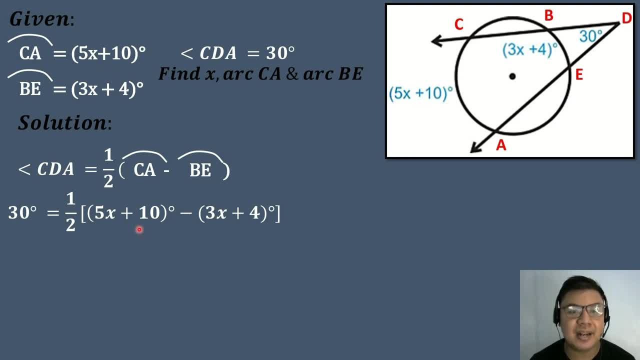 bigger arc is equal to 5x plus 10, minus the value of arc be is equal to quantity 3x plus 4, and then bring down 30 degrees equals. bring down one half and then after that we will bring down 5x. bring down positive 10 and then 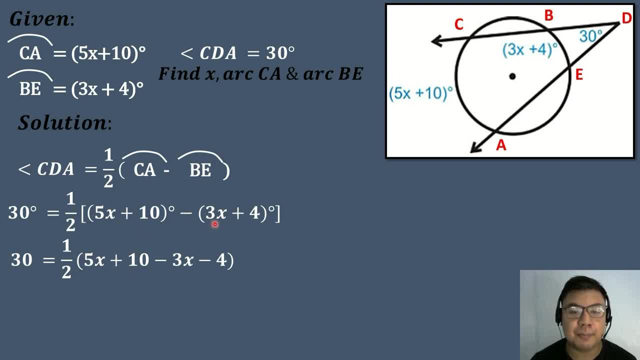 we will distribute the sign. so negative times positive: 3x will be negative 3x. negative times positive: 4 will be equal to negative 4. and then simplify again. so bring down: 30 degrees equals one half and then combine like terms: 5x minus 3x is equal to 2x. 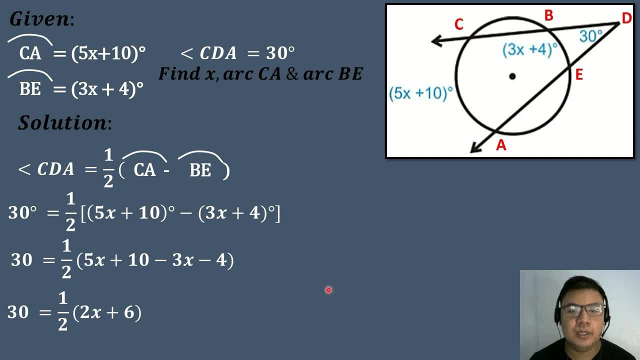 10 minus 4 is equal to 6. and then bring down 30 one half times 2x will be equal to x. one half times positive 6 will be equal to positive 3. and then after that bring down 30 positive 3, transpose it will become negative 3. so x is equal to 30 minus 3. so the 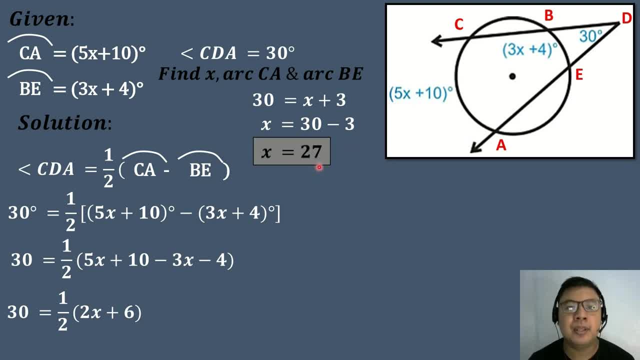 value of x will be equal to 27 and then after that to get the measure or the value of arc ca, we will substitute the value of x to the equation. arc CA is equal to 5x plus 10 degrees, so substituting the value we have 5 times 27. 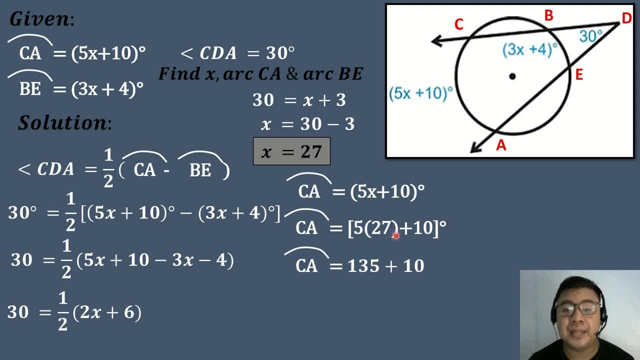 which is equal to 135, and then being down plus 10. so 135 plus 10 will be equal to 145 degrees. so the measure of the bigger arc, which is arc CA, is equal to 145 degrees. and to get the measure of the smaller arc again, we will substitute the value of x, which is equal to 27. so we have